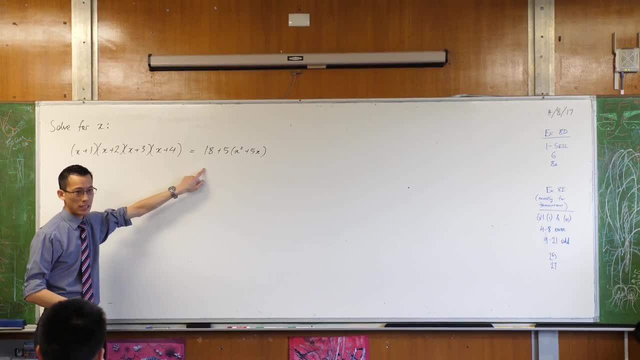 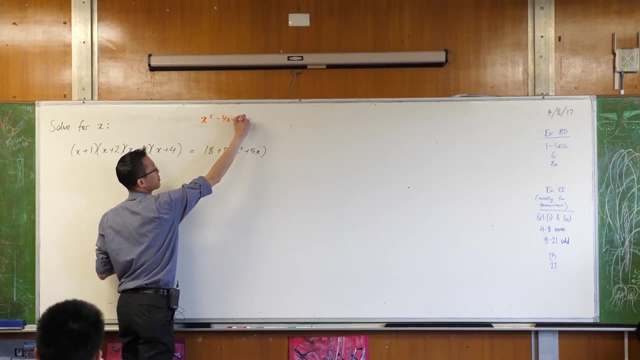 5x squared plus 25x plus 18.. I'm going to give you a suggestion. Do you remember? I think yesterday, one of the quadratics I gave you was- I don't know something like this right, And we looked at it and we immediately saw, without any computation, don't bother factorising this- and the big flashing clue was the 7, right. 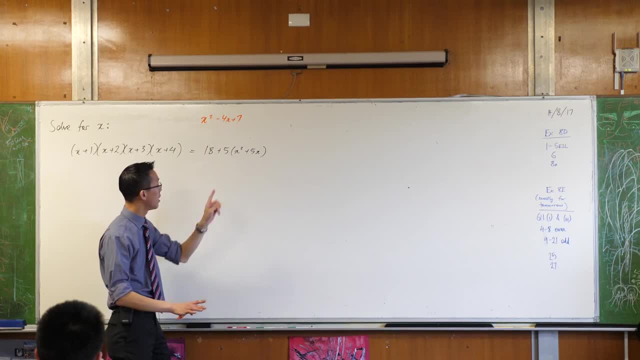 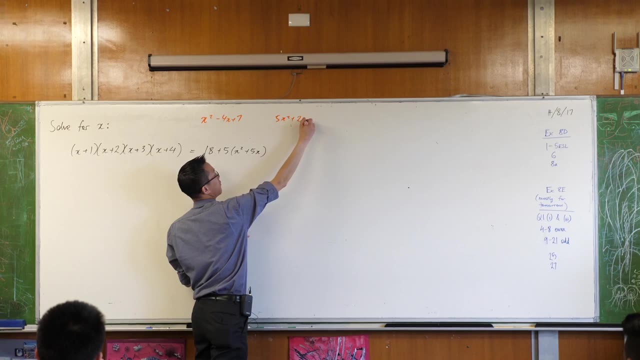 Now this is not the only clue that should tell you factorising is a bad idea. If we, just because it will just take us one second, if we just expand this, watch what happens: 5x squared plus 25x plus 18.. Is that right? 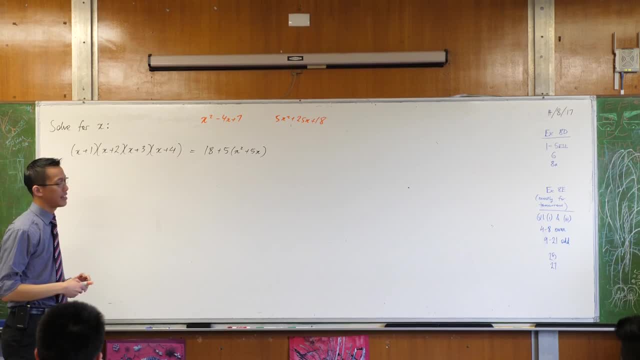 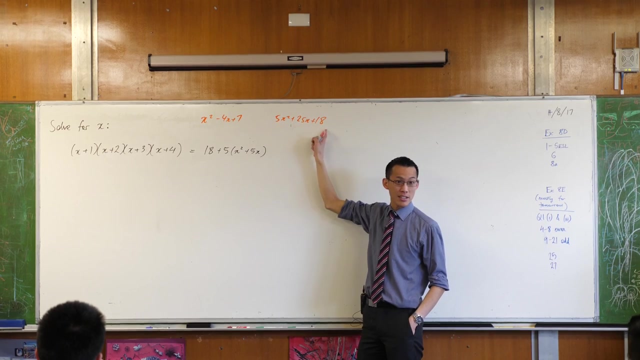 Now, 5 times 18 is 90? 90.. 90, 25,- hmm, Doesn't take you very far, does it? And here's the reason I know I need to have something that's going to multiply to 90,, right. 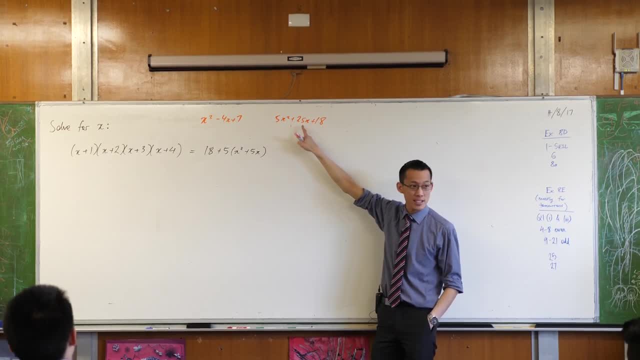 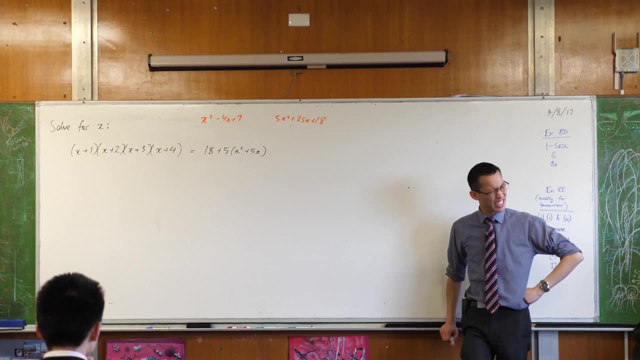 But you can see the factors here are going to have to somehow fit into this, but none of them do. It's not going to give you anything. So even if you went down this alley, it doesn't get you very much progress, okay. 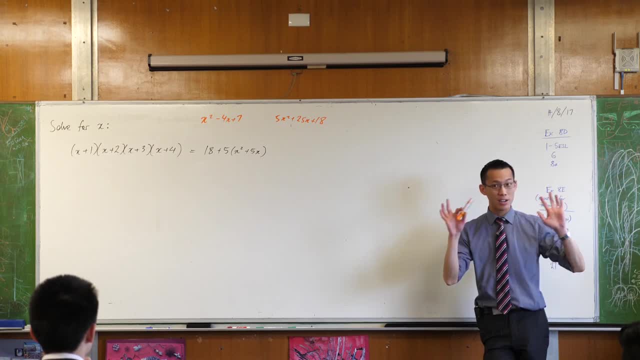 So, again, I'm going to rewind and I'm going to give you that clue I said at the beginning, which is that this comes in an exercise about equations that are reducible to quadratics. okay, Now, this does sort of stick out, doesn't it? What's that doing there? 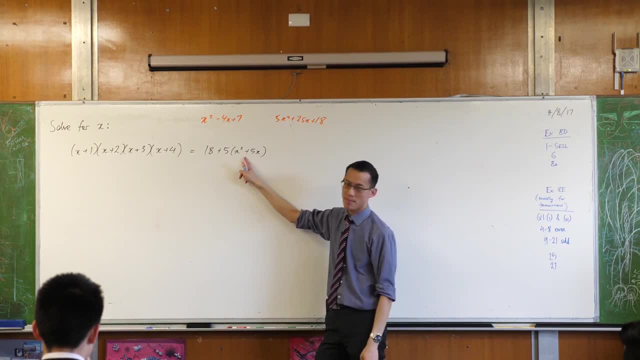 Okay, this at least seems like someone made that up. but why is this separated out? That's why, Oh, didn't seem like a bad idea to expand it. okay, This thing here is the key. This guy is hiding over on the left-hand side. 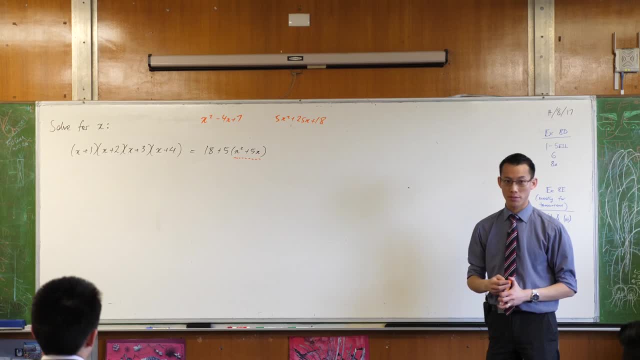 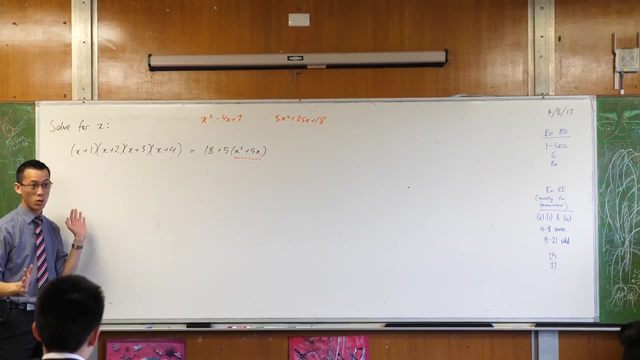 Actually it's hiding there twice. We just need to be able to find it. Now you can see if we did expand this. if we did expand this, expanding the whole thing would give us a quartic. okay, But you could expand them partially. 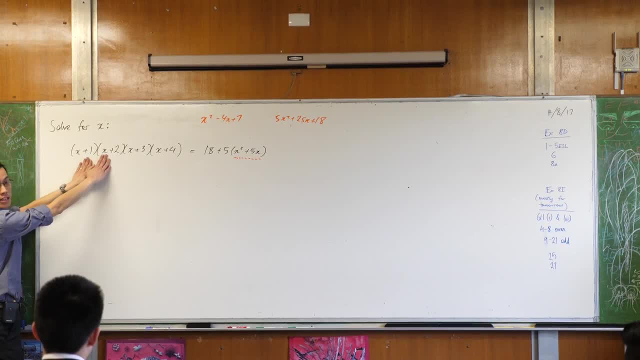 You could extend, say, pairs, For instance, if you expanded these two, just these two, forget about the rest of them, okay. What would you get? You'd get x squared plus 3x plus 2,, wouldn't you? 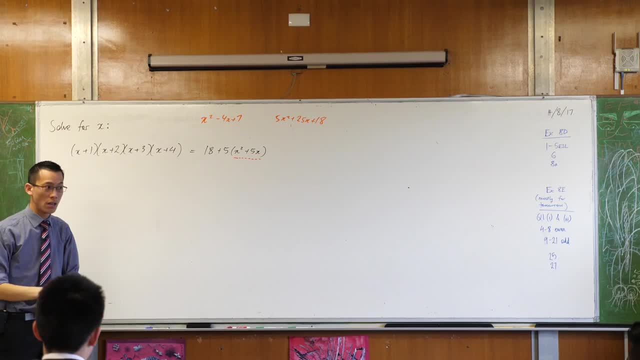 Because, look, there's the pair of numbers: They add to 3,, they multiply to 2, so that's what you would get: x squared plus 3x plus 2, that's easy to deal with, but it doesn't have anything to do with this, right? 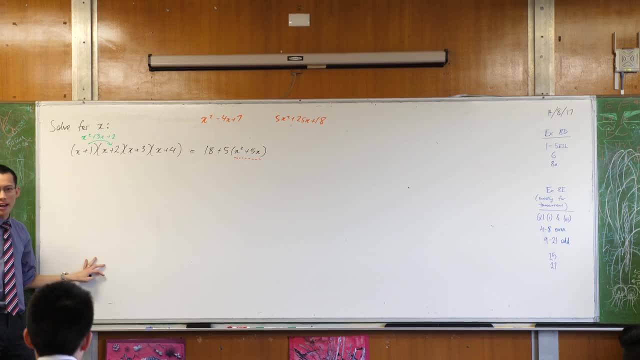 And of course that's because this is not the only pairing up that I can do over here on the left-hand side. There are other things. There are other things that I can pair. For instance, instead of pairing up the x plus 2 with this guy. 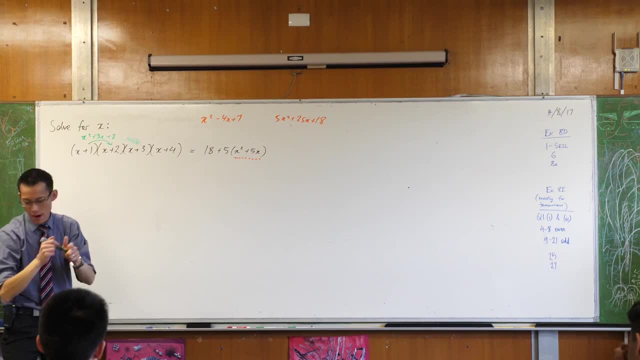 let's try pairing up the x plus 2, that's a bad choice of colour. let's pair up the x plus 2 with this guy. What will I get? You should recognise this. This is my favourite quadratic function of all time, okay. 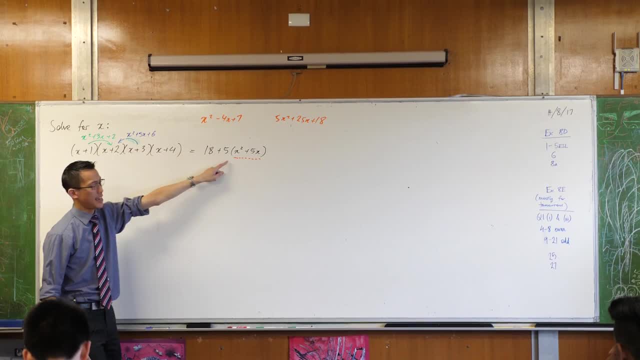 You're like: oh wait, this thing, this thing is not the same, but it's clearly related to this, isn't it? And in the same way, if you have a look at what's left, if I use these two up, expanded those, then what I'm left with is these ones. 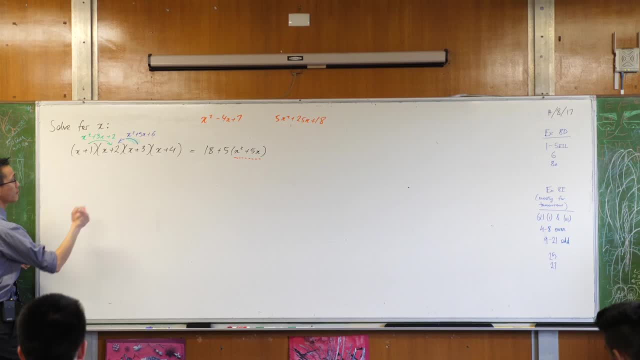 What do they expand to? x squared plus 5x plus 4.. Are the gears turning yet? Do you see what we've done here? We have a clever choice of what's over here on the left, because you can choose. This is the most important part. 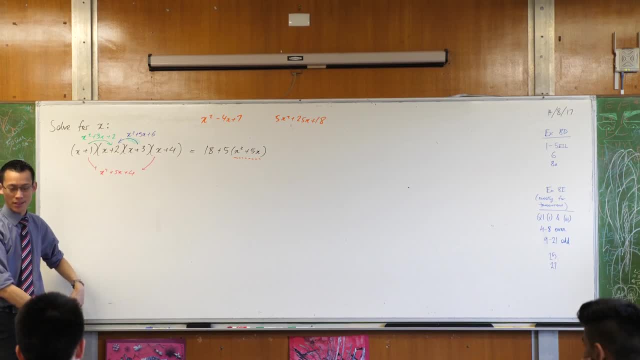 The most important part in a maths problem is the choosing, not the actual computing. okay, If we choose these well, on the left-hand side, I'm going to get this. what was the first one? you gave me Plus 6, that guy from the middle. two. 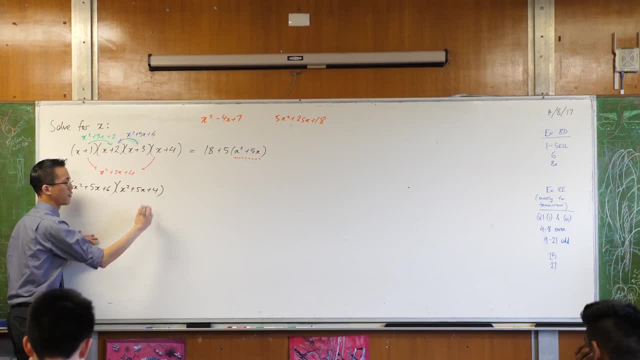 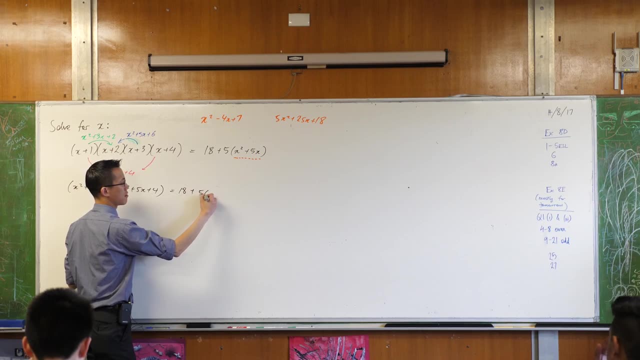 And then this from the ends. Does that make sense? So this is the same as the first line, and what I have over here doesn't need to change. okay, So now can you tell me a substitution? What should I? let's introduce a substitution like u. 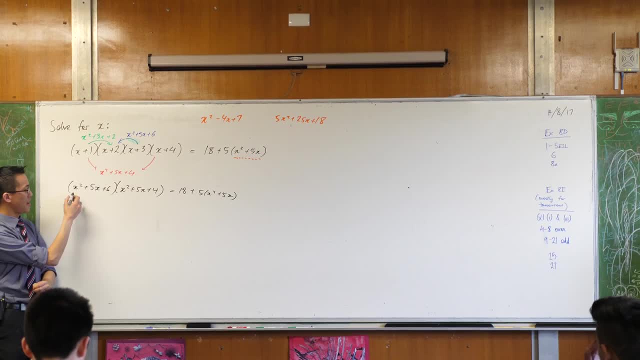 What should u be equal to? Yeah, there he is. 1,, 2,, 3. He appears all of those times. So if I let u equal what you just told me, tell me what to write on the next line. 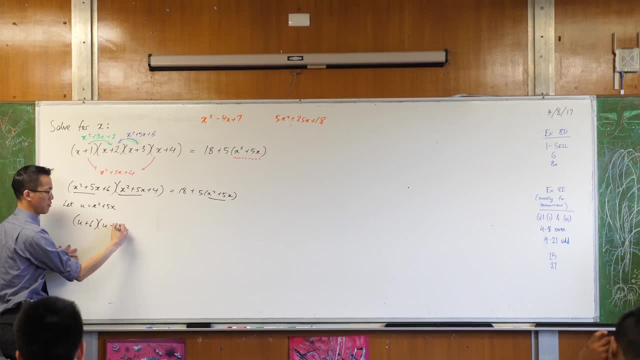 u plus 6,. u plus 4, equals: what have we done to our quadratic? We have reduced it to a quadratic and I reckon you guys can take over from there. Okay, in fact, can you see what you get? 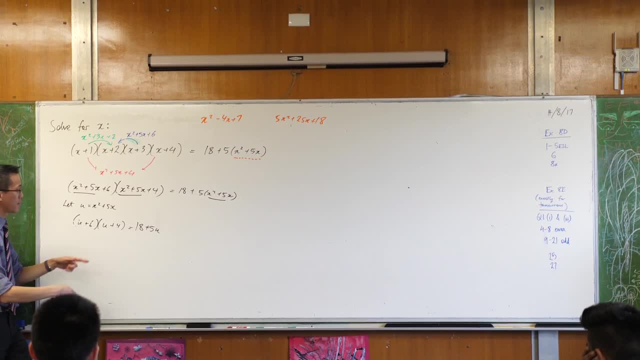 You're going to get a solution for u And then you're going to go to the next step because you want to go back to x's. Okay, any questions? After what exercise did you start? 8, uh, Jake d.